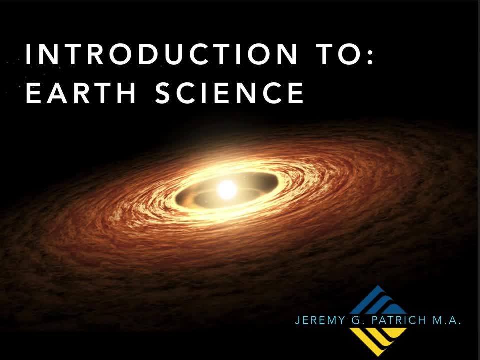 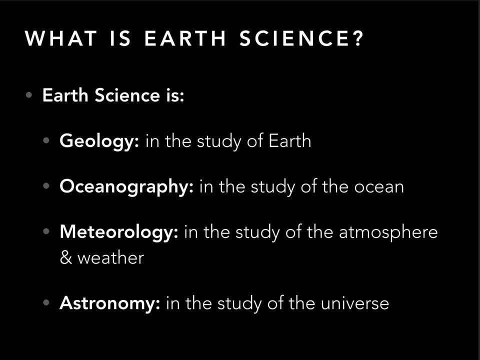 They don't want to take geology, They don't want to take oceanography, They don't want to take meteorology or climate sciences, They don't want to take astronomy. So they think, oh, Earth Science, This will be an easy one to jump into. Well, surprise, surprise, Earth Science is all of those things lumped in together. We learn about the geology, or study of the Earth. We learn about oceanography and the study of our oceans, meteorology, understanding our atmosphere and weather, And we also learn about the study of our universe and our place within the universe. So Earth Science covers a lot of different pieces. 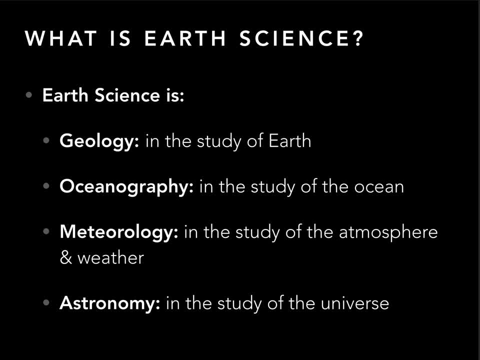 Each one of these is a normal 16-week course at most institutions, So we have to somehow merge all four of these topics into a palatable system. So it's going to be exciting to know that we get to talk about so many different things. 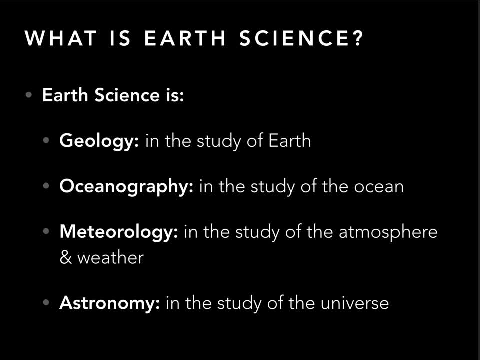 We're going to be able to talk about everything from climate to clouds, to volcanoes, earthquakes, plate tectonics, solar nebula- I mean pretty much everything you can think of is probably going to be brought up into this course. So it will be exciting and does cover a lot of content, But we'll make it palatable, We'll make it easier to understand, Trust me. So let's look at each one of these a little closer. 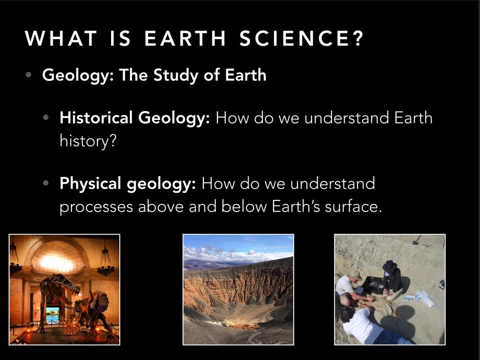 So the first one is geology, the study of Earth. So we have two pieces. We have historical geology and physical geology. So historical geology is really: how do we understand Earth history? So as an example you'll see, there's a photo down here. This is me and some colleagues. We're actually excavating a left leg of a woolly mammoth that dated about 10,000 years ago in the eastern Sierra. 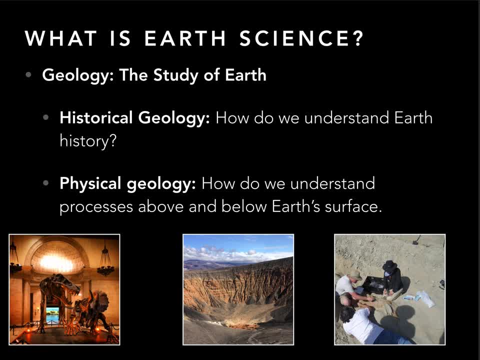 So we started looking at some of the underlying geology, the sedimentology, understanding the environment in which he would have died in- because he actually died on a beach ridge. So we start learning about the past. Again got to do your cliche Instagram photo of the museum and actual history, But we can understand the history of the fossil record, geologic time. 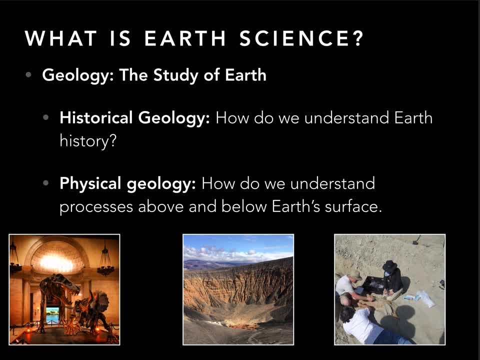 Well, why is that important? Well, because once we understand that system, that evolution, we then bring into physical geology. How do we understand the processes above and below the surface and into the future. So we get to then look at this landscape in the middle. This is a photo. 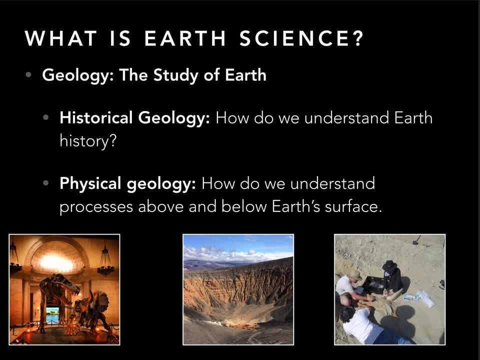 I took of Ubehebe Crater in Death Valley National Park. It was a volcanic area. They're craters themselves looking at steam vents. but looking at its past allows us to understand geothermal activity in other locations, to learn about its future. The next one we'll look at is oceanography. 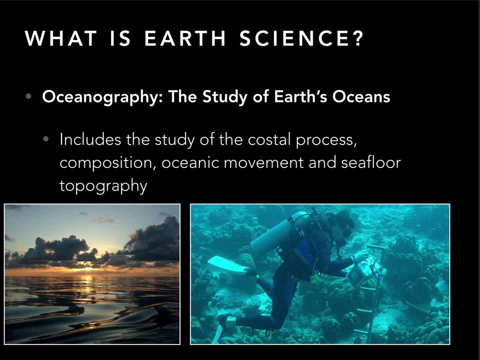 This always excites me. I have a lot of friends who get to teach this course and the first thing they say is: students become often discouraged when they enroll in this course because they think it's about marine life. Well, that's marine biology. This is still an exciting course because 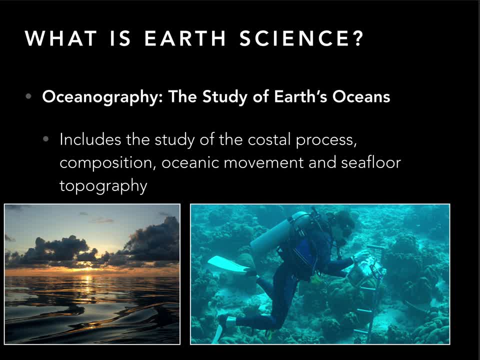 it teaches you the coastal process, composition of the ocean. We learn about oceanic movement and seafloor topography. We learn about steam, the vents, volcanic vents. We learn about volcanic ranges and arcs, and so there's a lot more in the study of oceanography than just whales. 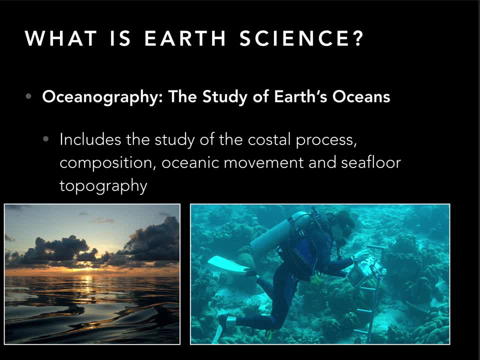 and dolphins. So we get to learn about the environment they live in. We get to learn about how the ocean interacts with our planet. and well, how do the oceans interact with our greater source, perhaps even looking at astronomy in that sense? Well, you know, we're learning about what? 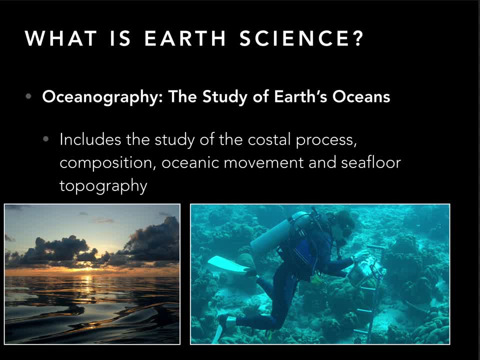 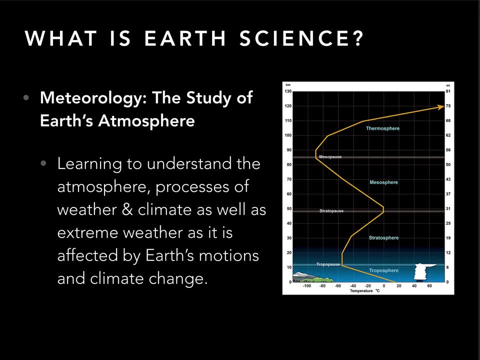 oceans are able to absorb, looking at greenhouse gases and things along. that It's really an exciting portion of this course, Moving into meteorology- really it's atmospheric sciences. How do we look at our planet's atmosphere? We acknowledge that we have four dominant layers. 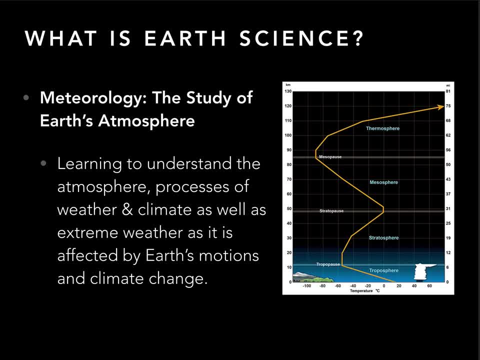 topospheres, where all of our weather occurs and where we live. Then, above that, we have the stratosphere, the mesosphere and, lastly, the thermosphere. So learning to understand the atmosphere, the processes of weather and climate, as well as what extreme weather might be. 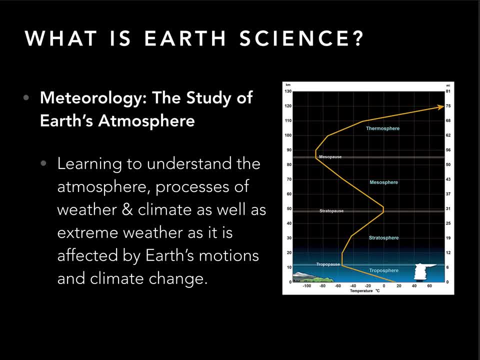 especially as it is affected by Earth's motions. looking at our interaction with sun and seasons, looking at even climactic change, even human-induced climactic elements, you know greenhouse gas contribution and what is the long-term effect. So really learning 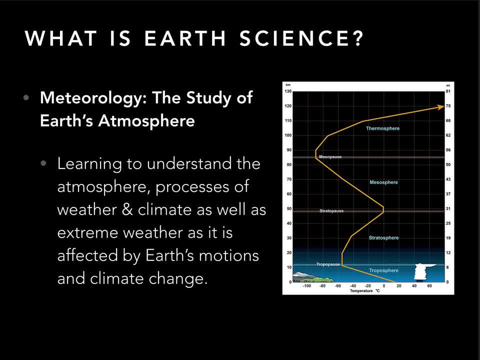 the difference between day-to-day weather and long-term climate. We'll spend some more time talking about that, but you know, weather is the day-to-day: It's hot, cold, wet, dry And climate is taking at least 30 years of data and creating a general statement and saying well. 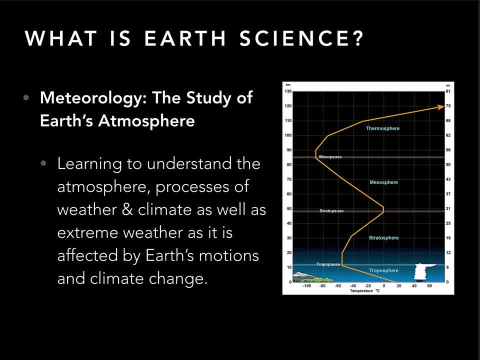 the climate in, you know, Las Vegas in July is generally hot. Is it possible that it can rain in July in Las Vegas? Of course it is, but that doesn't mean that, you know, generally it's going to be hot and dry. 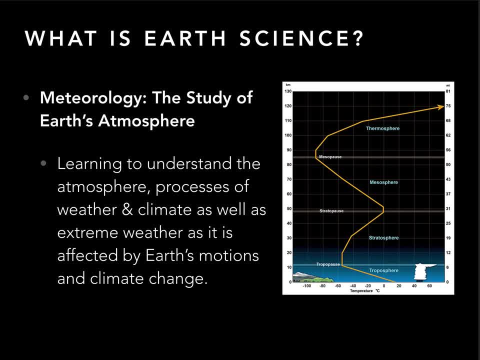 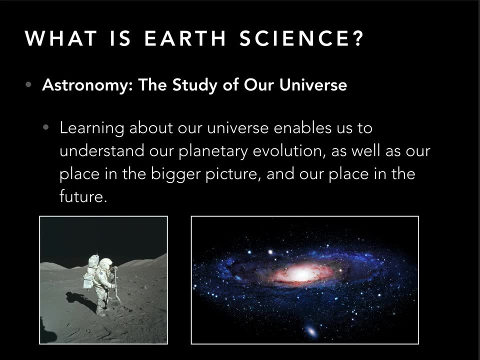 We have this 30-year value of data that projects, that And by understanding that, we're able to project and predict tomorrow's weather and maybe even tomorrow's climate going forward long-term. And the last one that we introduce is astronomy: the study of our 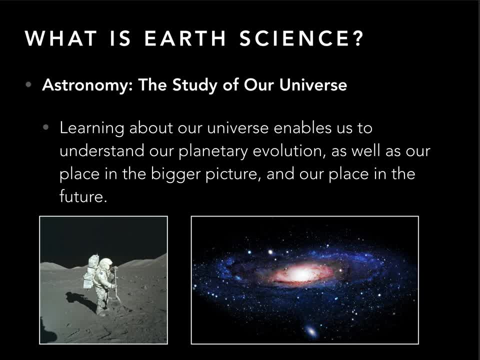 universe. So learning about our universe allows us to understand our personal planetary evolution. Where did Earth come from? Where is it going? You know, what are we starting to observe about the future? Well, we have, like very philosophical you know, to understand yourself, you have to understand the. 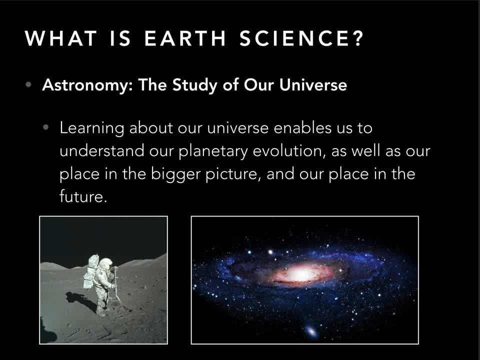 environment around you, because that definitely is a reflection of what you are. So when we start to learn about other locations and watching the birth of stars and planets, well, what does that mean, you know, for our future here on Earth? Why are we, you know, striving so hard to find? 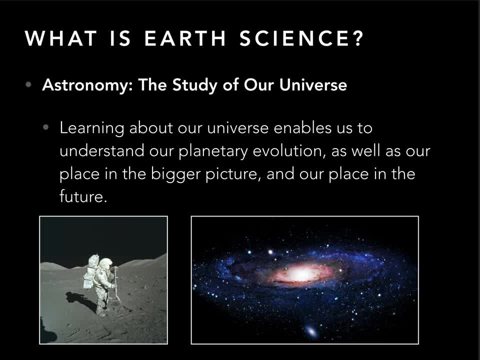 planets that can allow life to thrive. You know we're trying to see if there's anything else out there, but why does that intrigue us? Why do we have so many television shows and movies and sagas that are about us? Why do we have so many movies and sagas that are about us? Why do we have so many? 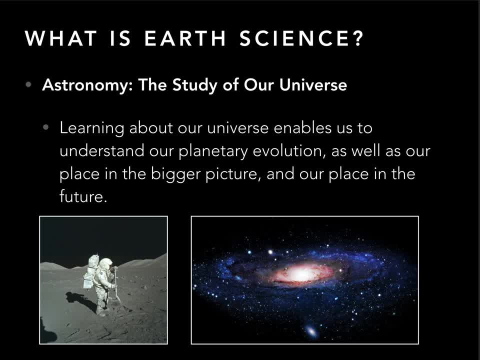 episodes and shows that are about the space and what's out there and how far and vast it is and how much more we continue to learn about it And hopefully we'll even get to cover — is Pluto really a planet or not? Why do people think it's not? So, nonetheless, let us continue So moving. 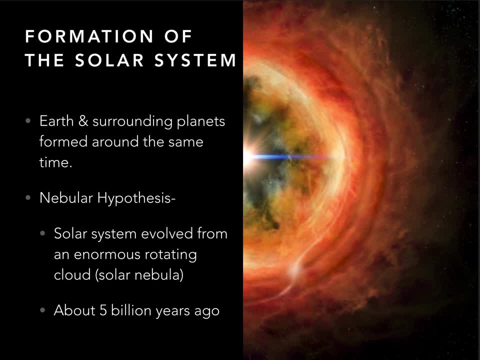 So moving forward. so we're going to introduce the formation of our Solar System, Earth and the surrounding planets formed around the same time, Geoemощ, Hmmmm, long-term scheme. You know the process was a large — what we have is a Nebula Hypothesis. The Solar System will point at any of the 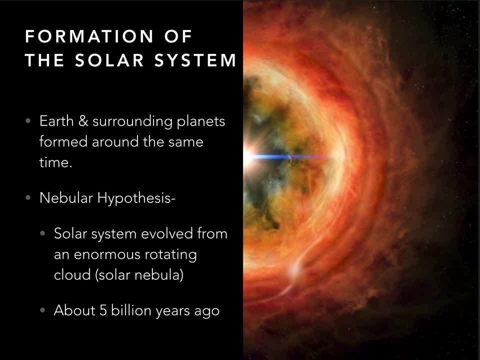 planets in the sky that exist outside Earth. There will be a shape, license or form that'll Allah will be able to accommodate. Let me give you some clues about, let's say, in terms of what will be the chance that whatever happens in the future, and then one or the other planets that will actually change about. 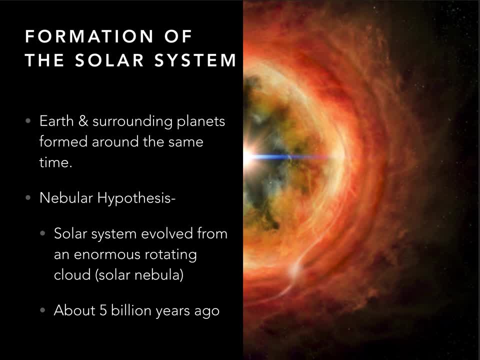 the solar system evolved from an enormous rotating cloud, or a solar nebula, And that was about 5 billion years ago, when all the matter and mass was available for this to occur. Well, after the formation of this nebular hypothesis that we bring us into, 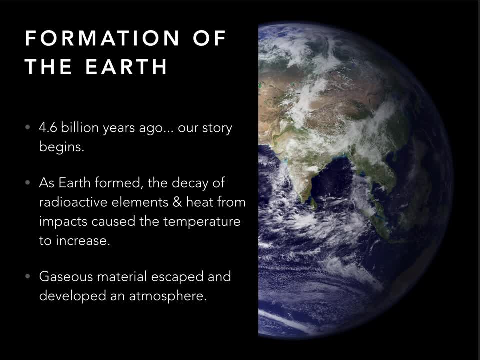 we can then talk about the formation of the Earth. The Earth planet itself is about 4.6 billion years old. That's when our story begins, once all that particulate matter was able to merge together and make a planet. So, as the Earth formed, the decay of radioactive elements and isotopes from the center of the Earth produced heat. 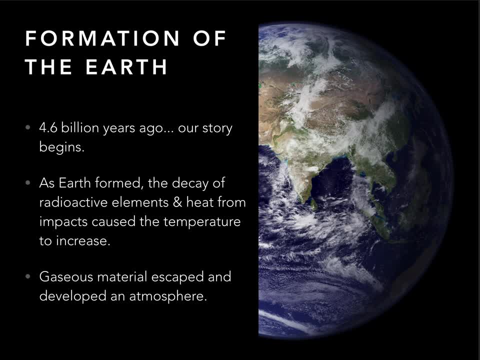 That ends up creating also the decay of the material on our surface. when it was still a molten planet, It caused the temperature to increase. This gaseous material escaped and developed a basic atmosphere. Why are atmospheres important? Well, atmosphere keep out asteroids, meteors, particulate matter from extraterrestrial matter. in that sense, 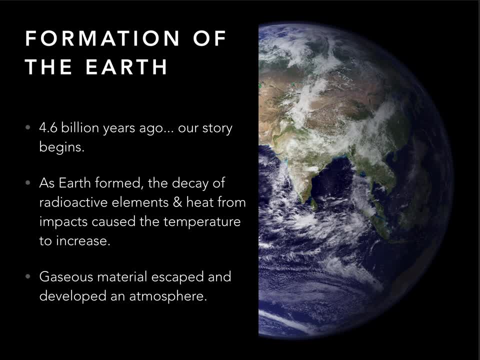 But also trap gases in, And that's important because we want to be able to trap in oxygen, Because that allows us the ability to survive. We'll learn a little bit more about where our planet, where we got our oxygen, Where we received most of our water. 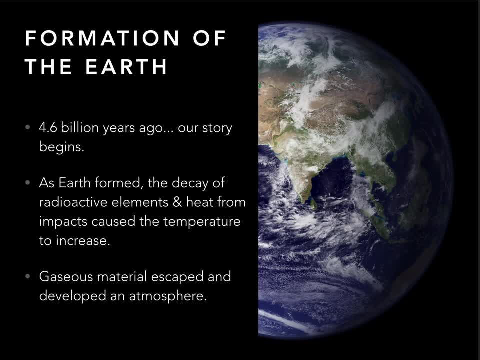 And we'll learn more about that in the future. But it's just to understand the formation of our planet. We're looking at a very, very long story. It's almost- It's almost unbelievable for us to try to imagine what 4.6 billion years is. 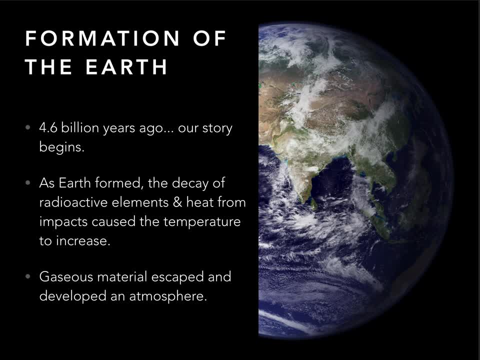 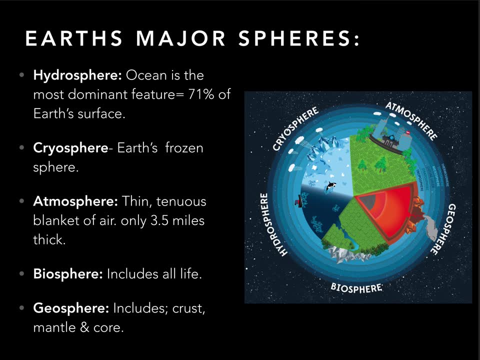 We'll learn a little bit more about that when we learn about geology, But nonetheless, big big story, We actually can divide our planet into quote-unquote spheres, Meaning, you know, realms, if you will. So I like this diagram. 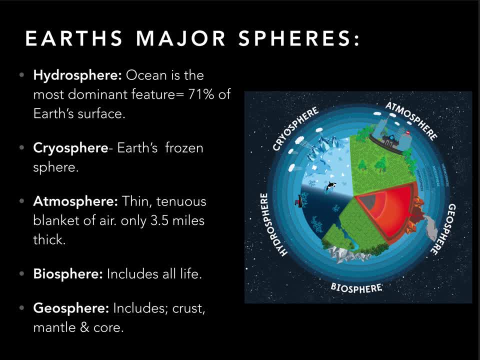 We often merge the hydrosphere with the cryosphere, But I label them as separate things just so we can talk about them that way. So the first one is the hydrosphere. That's water. Anywhere there's water on the planet is involved in the hydrosphere. 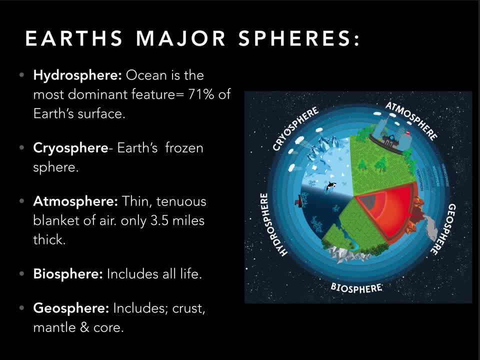 So think, Think back. when you learned about the hydrologic cycle. It's You know this is. We're talking way beyond just evaporation, condensation and precipitation. When we start looking at the hydrosphere, we're going to learn about transpiration. 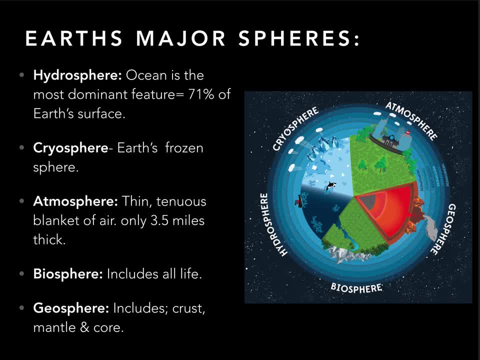 How water works with plants, How it works with storage, How it looks with underground And looking at different elements like that Moving into the cryosphere, Adding in the element of ice. Where is it stored? How much is there? Why is it there? 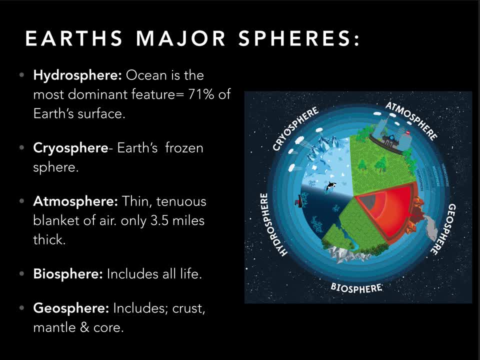 Is it getting bigger, Is it getting smaller? Is it thick, Is it thin? So, understanding its process, We'll also be discussing basic geomorphology, Looking at how the hydrosphere and cryosphere, water and ice itself carve and shape our planet. 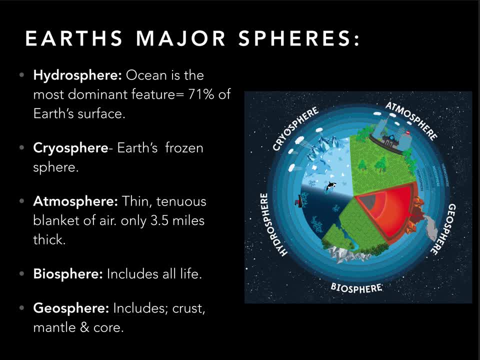 We also look at the atmosphere again. That's another one of our spheres. It's very thin, It's only about three and a half miles thick, Yet it's able to protect us from everything, Which is really really, really important. 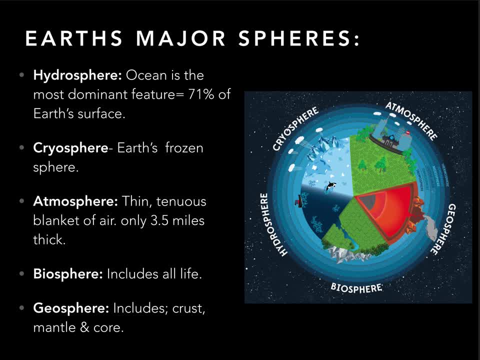 It blocks out bad Negative and bad UV radiation that would otherwise cause us to burn. It keeps us at a relative temperature Versus fluctuation of very cold or too hot. We also will introduce the biosphere, Which is all life, That's everything from plants to you and me. 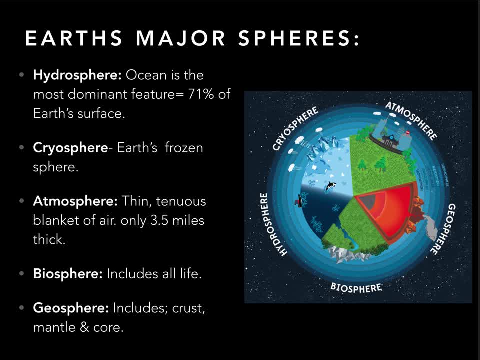 And then we also have the geosphere, Which is all rock. So we have these spheres that we introduce To kind of, you know, make it more of a realm. I don't know, I learn better when things are kind of chunked together. 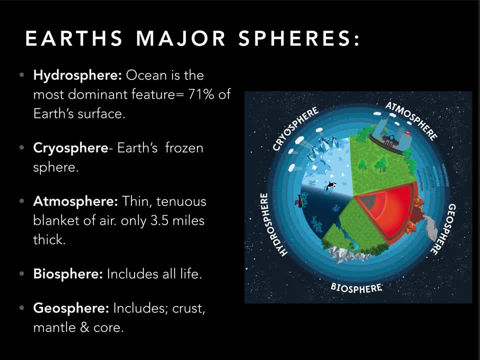 When I can see that, there's Okay. So these are all the things within the biosphere, These are all the things within the geosphere, These are all the things within the atmosphere. So again, I like this little diagram. It kind of gives an element. 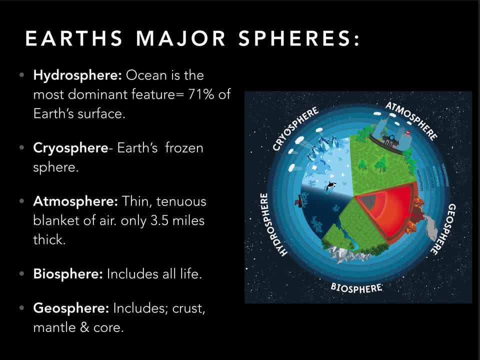 Geosphere. We can see there's plate and tectonics involved. There's layers of the earth. We can see there's volcanics. We can see within the atmosphere. You've got all your different layers and special zones. So I just kind of like this type of. 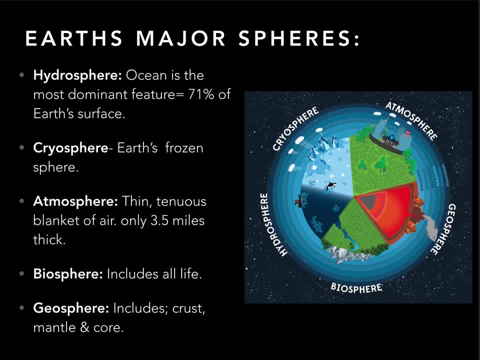 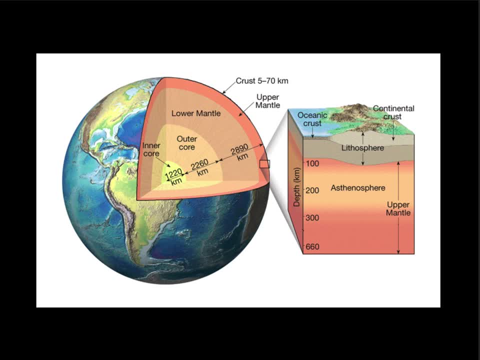 What I call putting it together. How do we put everything together? Well, since we mentioned it, We'll talk about it. You know, we understand, that we live on a dynamic planet, Constantly changing. You know, understanding that we have these different layers of cores. 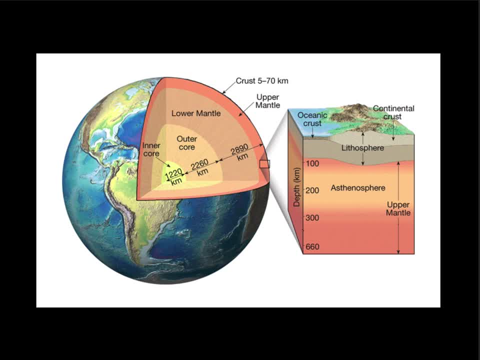 When I think of the layers of the earth, I also will talk about this in atmospheres. I think of salad dressings, Like those homemade ones Where, if they sit too long, they separate. So they separate based off their densities. Well, what if we could observe that idea here? 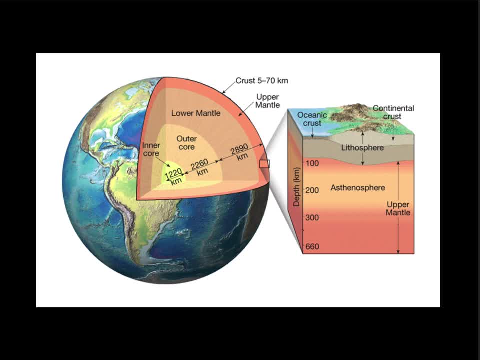 Looking at both densities and temperature. That will allow us to understand why we have these different layers within our earth, Moving from the inner core to the outer core, to the mantle. Then looking at the asthenosphere, Which is a plasticky zone that protects us and allows us to move around. 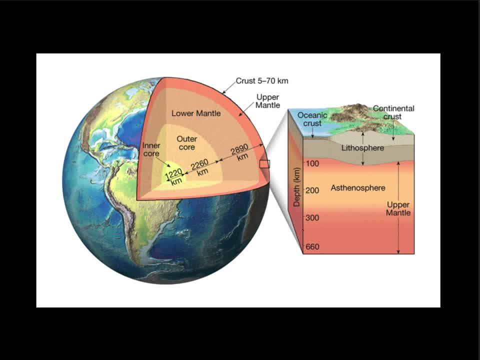 The lithosphere, Which is the rock material that we live on, And then we have our crusts, Both oceanic and oceanic, Oceanic and continental. We'll also learn the differences between these crusts. Oceanic crust is predominantly basalt. 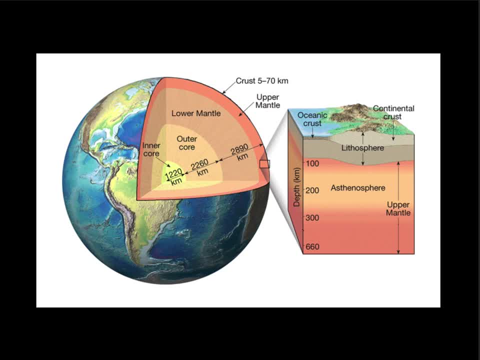 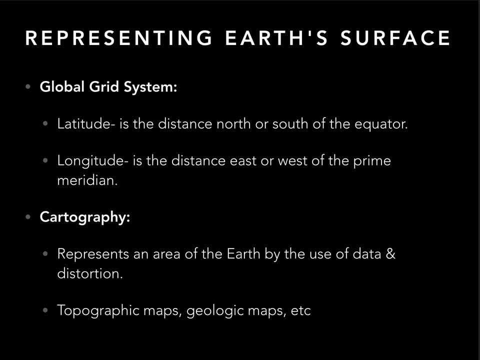 Continental crust is predominantly granite. Very different types of formations, Both igneous rocks, But both formed under very different environments. Another thing we can talk about is: Well, how do we look at the earth's surface? Well, we've got global grid systems. 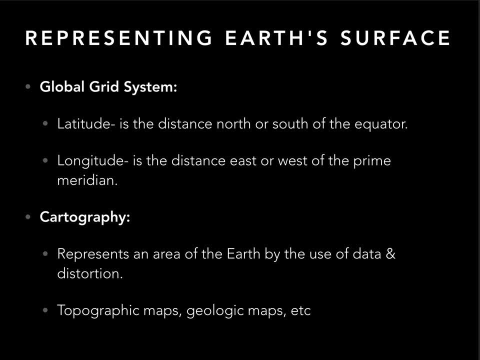 We look at the value of latitude, Which is the distance north or south of the equator. When I think of latitude, I think of pizzas, The metal pan they cook them on, So all kinds of different sizes, Yet they're all circles. 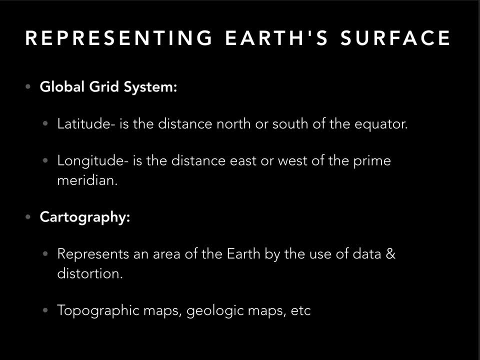 Well, that's kind of what latitude is. Latitude is the distance north or south of the equator, But drawn all the way around. So they're lines, that kind of work themselves as discs around the earth. Well then you have longitude. 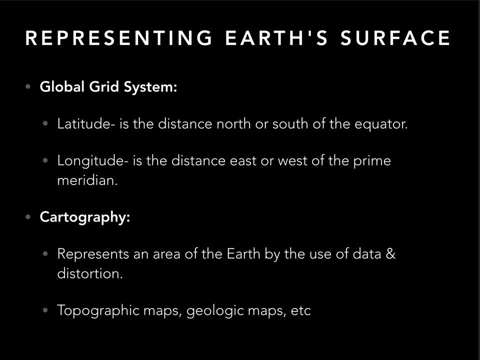 Which is the distance east or west of the prime meridian. Well, longitude is like an orange, So they intersect at the north and south poles But create a meridian or a half circle. So because you have these two different lines That are running in different directions, 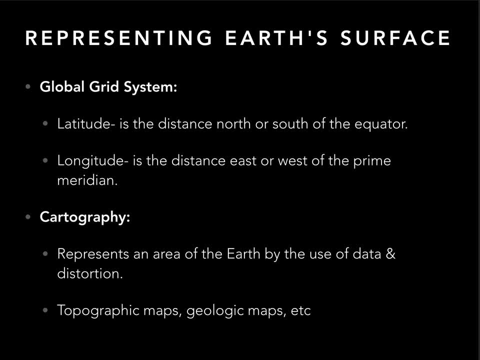 We can create intersecting points, Which is going to be part of your grid system. We'll talk more about that later. We also look at cartography. That is an art in its own. It represents an area of the earth By using data and distortion. 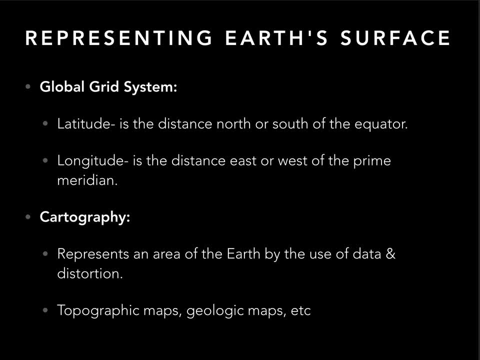 We look at topographic maps, Geologic maps. How do we view the landscape? Most of you probably don't even own a map Or a Thomas guide or anything like that, But you have experienced true cartography, Especially if you play video games. 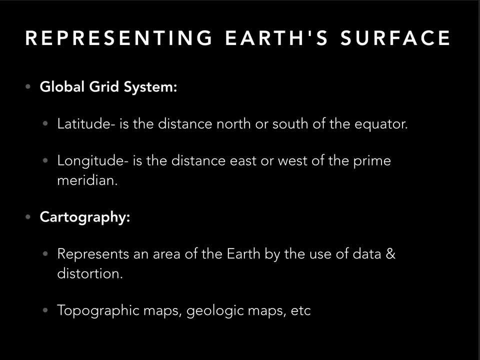 A friend of mine works for the World of Warcraft, And her job as a geologist Is to help them design their landscape And to create a map That is believable to its consumers. You So, if you're playing these video games. 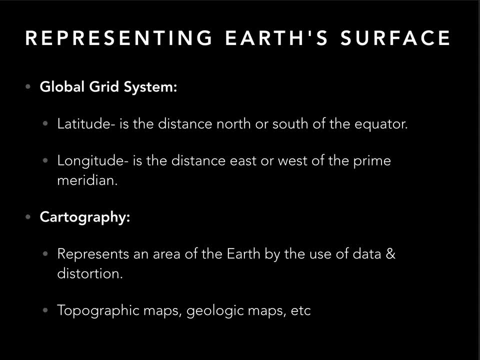 And they're in landscapes that have volcanoes And trenches And volcanic ranges, Everything in between. That's because it's been detailed by an earth scientist, Because we've been able to represent a landscape That is probably functioning. That's true, so that we can believe it. 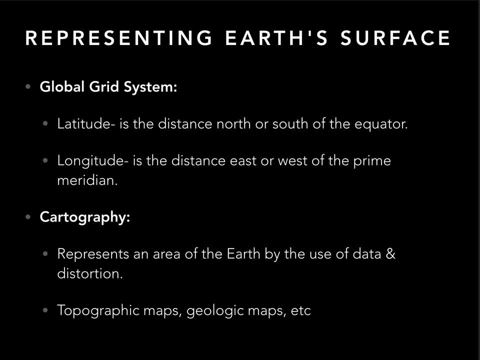 Because, let me tell you, If you play a video game In a landscape that did not make sense, The game will not make sense to you. Think about that. Have you ever played a game That you're looking at? I'll give you an example. 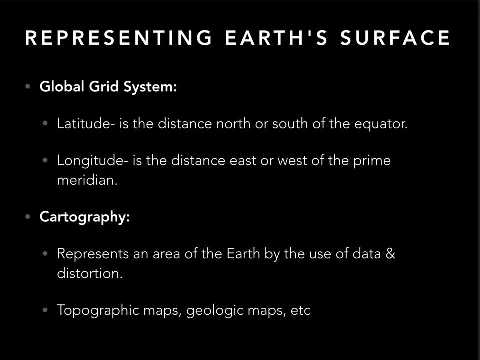 I knew a student who was part of a video game design program And they were trying to build this video game Where it was an island, A very small island, And the island was like a pie And it would be divvied up. 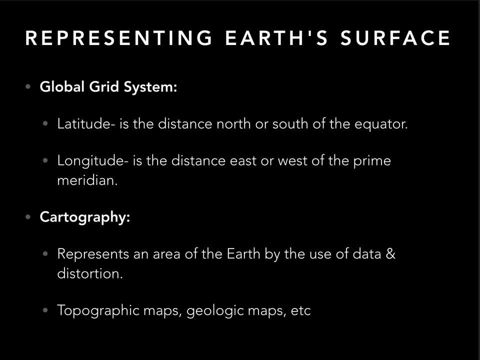 This is going to be the desert. Geologically, And looking at it as an earth scientist, The way they had it designed Was not going to work in a real environment, And so therefore it doesn't make it very believable. So how do we interpret it? 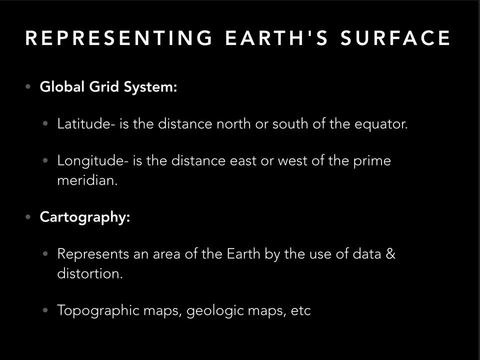 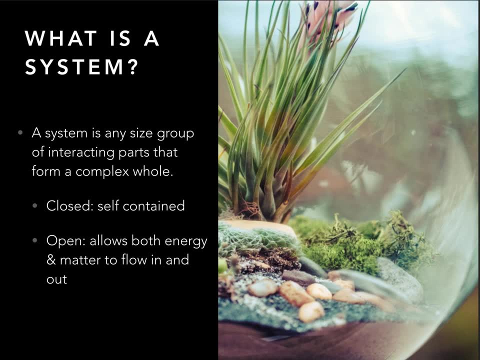 How do we make these locations believable? And that's understanding the process And understanding the spheres And how they interact with one another. Then we'll look at systems. Well, what is a system? An institution is a system Of people that work together to make progress. 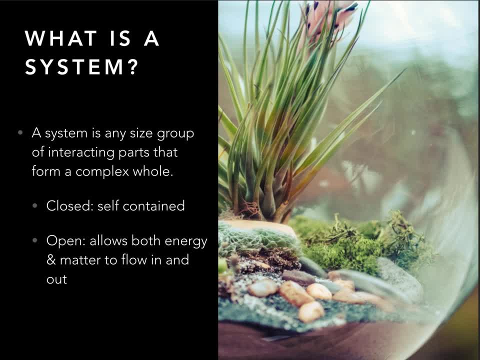 So a system is any size group, Interacting parts that form a complex whole. So you, as a student, are part of a system, A bigger system, Because, yes, you're a student And I'm an instructor, But I'm still going to learn from you. 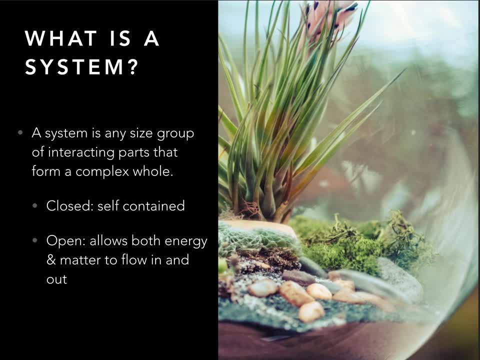 We're supposed to work together To create a bigger resolution And to create more information and more data. Now there are two types of systems. There are closed systems, Which means they're self contained, Which means they don't take anything in. 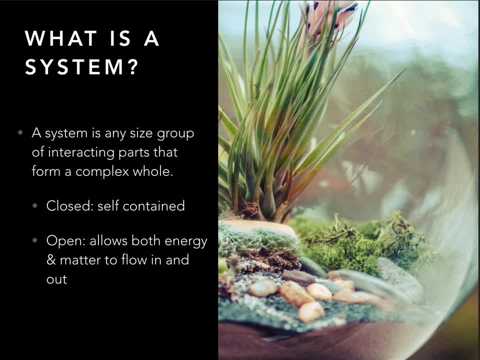 And they don't put anything out. And we also have open systems. So we have closed systems And open systems. Now I bring this up because What are some earth systems, What are some systems that you think could be open or closed? 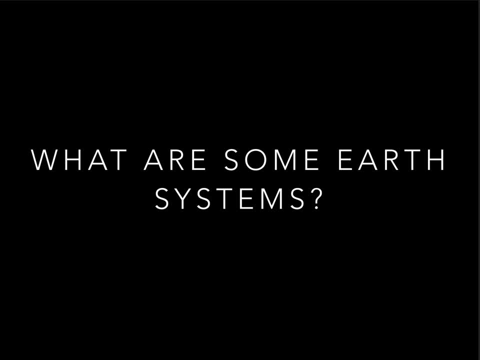 In fact, I'll give you a hint. A lot of people argue that there's no such thing as a closed system. Right, You know, Let's think of an open system. Vegetation: Well, Plants require sunlight, They require that short wave radiation. 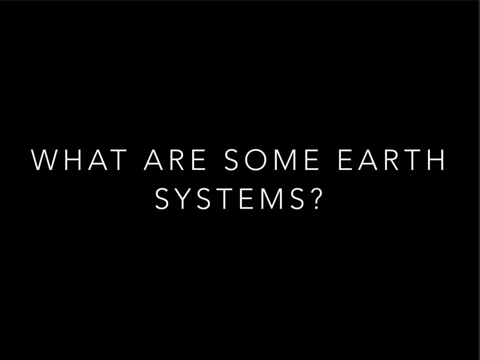 In order to go through photosynthesis, They also require carbon dioxide, Because then they produce oxygen, So they are taking in And putting out. You are an open system. You need food, So you can then gain the calories, Which then give you the ability to do work. 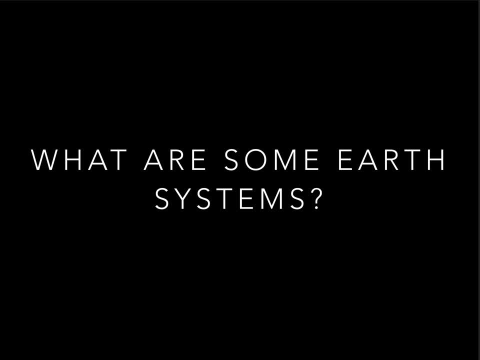 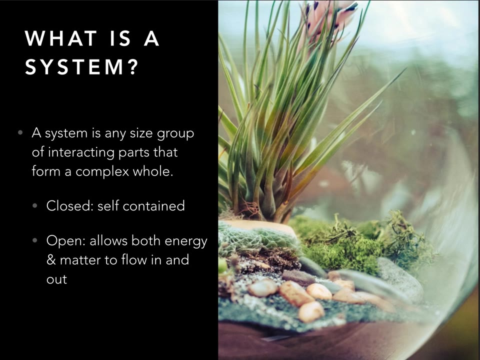 To have energy. So then, By having energy, You are able to move around and you produce heat, So you are also an open system. Often As an example, What about closed systems? People think that terrariums, Like this guy right here. 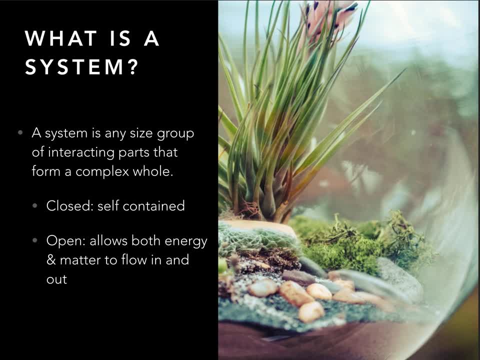 This is a closed system. You put the plants, You put everything in there, A little bit of water, You seal it, Put a cork in it And then it's done forever. Right, You never have to deal about it again. 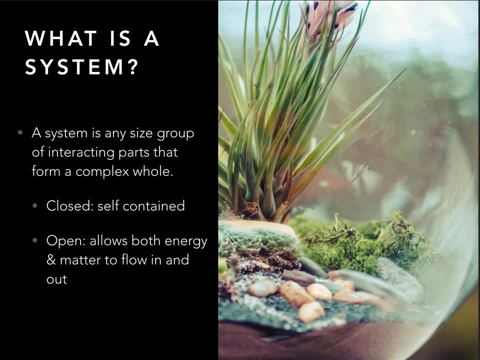 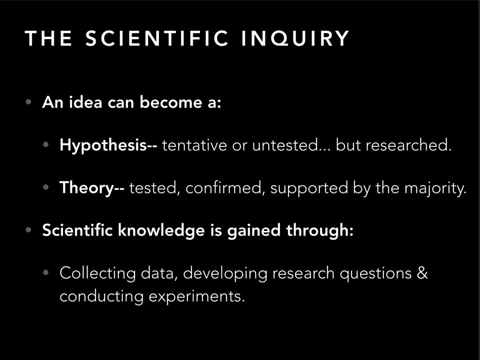 Well, But it still requires sunlight. So that's the argument: Well, it still requires sunlight, But everything else is trapped inside, So it's not able to be open. But is it really closed? Not with other closed systems. How do you do that? 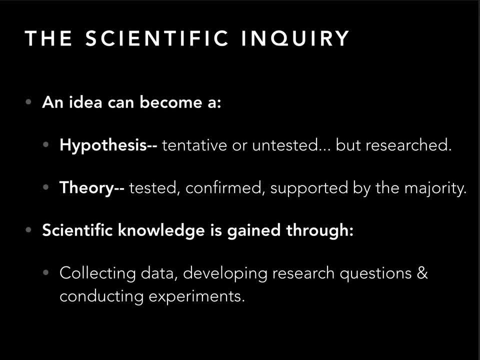 Well, we can use what we consider the scientific inquiry, Which is really a very important method, As anyone should be able to use this system. This is how we should think. We have an idea. That idea can either become a hypothesis, Which is tentative, or untested. 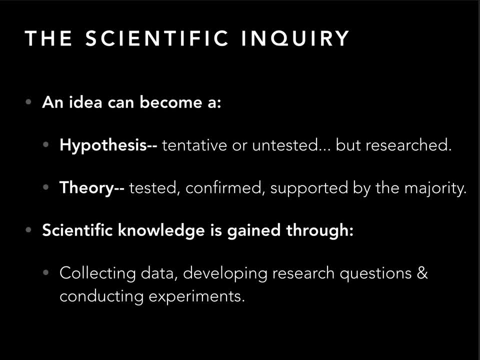 Or it will be a theory Which is tested, Confirmed and supported by the majority. So when people say, Well, I have a theory about this, They are actually not correct in saying that Unless it's been tested, Confirmed and agreed upon. 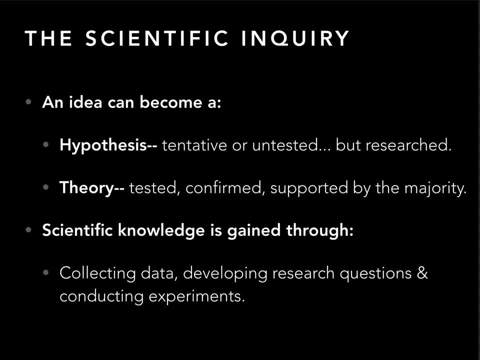 By the majority of people Who are also specialists in that topic. Then we are coming up with a hypothesis, Right? Well, I think that these are the winning numbers for the lotto. Well, that's a hypothesis. You don't have a theory for that. 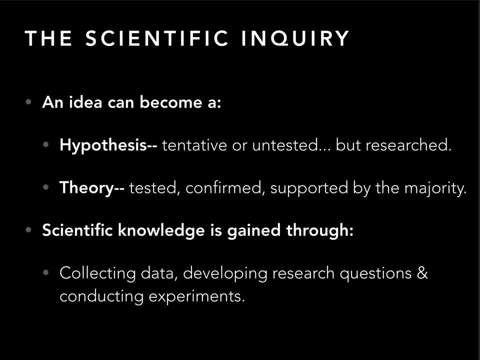 So when we talk about the theory of evolution Or the theory of plate tectonics, A theory means That word means it is. It is plate tectonics, It is evolution, We have confirmed it And it is supported by the larger group. 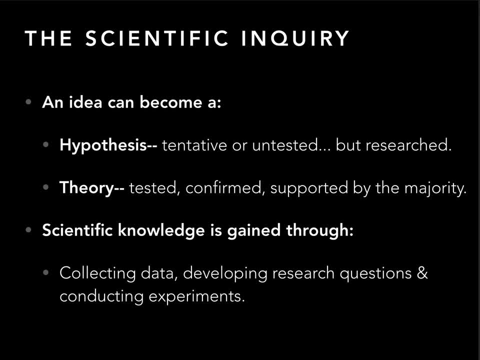 Scientific knowledge can only be gained By collecting data, Developing research questions And conducting experiments. So that is very, very important, Because often We as a society Jump to conclusions. We see something on social media And then we just believe it. 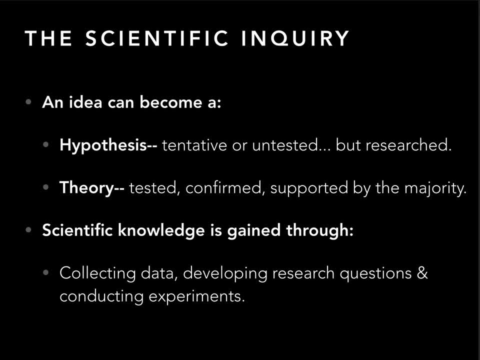 It has to be this. We don't question things We understand. Please explain to me. Think about: with any conversation People they say it on first dates- Never bring up politics or religion. But I don't think it is a bad thing. 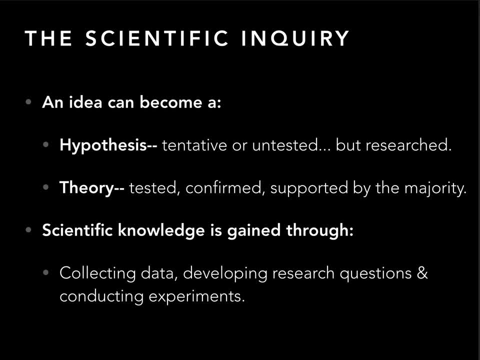 Especially if you want to learn. I want to learn about your politics. I want to learn about your religion. I don't think you are wrong And I am not going to argue if you are right. I want to learn And be able to ask the right questions. 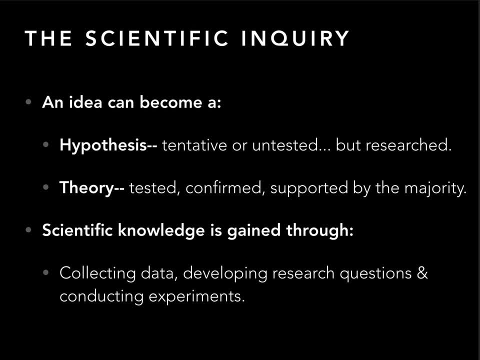 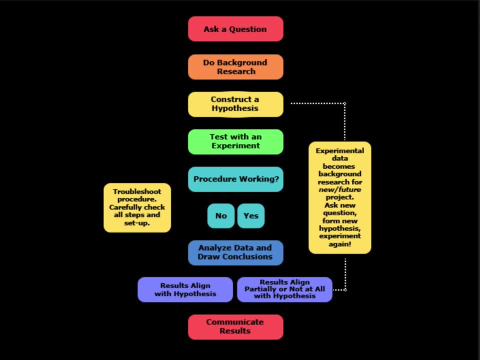 So I can understand what it is that you believe And understand what your methodologies are. So let's use this as an example. This is your classic, classic Scientific inquiry diagram. You first ask a question, Then you do research. After you have done research. 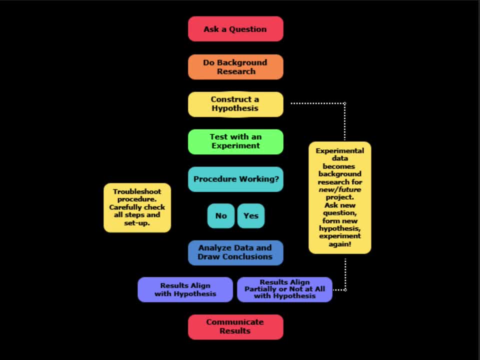 You construct a hypothesis, Then you work through it And when you get to the end, Then you can state that it is a theory. So Let's ask a question. I think that people Who are really tall Have to wear bigger shoes. 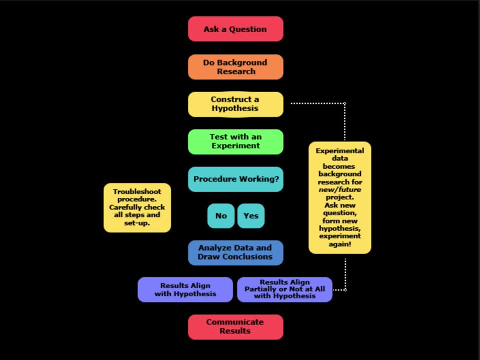 That is my thought. So I need to do some background research. Well, some basic background research. I could go to Nike for the weekend And hang out at the store And just kind of peruse people And go, let's see, Based on their height. 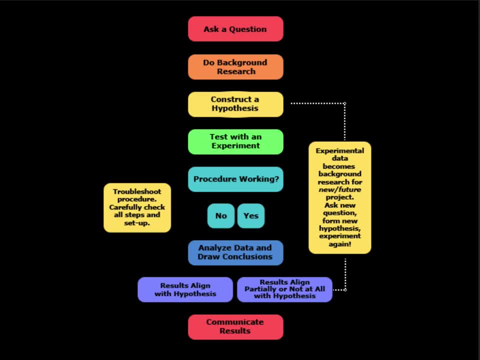 What type of size, What shoes are they buying? Are they buying these really big Size, 12 or 13 shoes? Are they buying more like a size 4,, 5 or 6.? So then, based on that observation, I need to do some data. 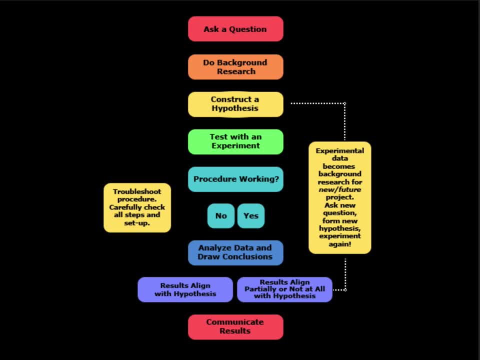 Formal data That is going to allow me to do some background research For either new or future project. And then I need to start asking questions So I can form it even better. So I am going to move down forward. So I am now here. 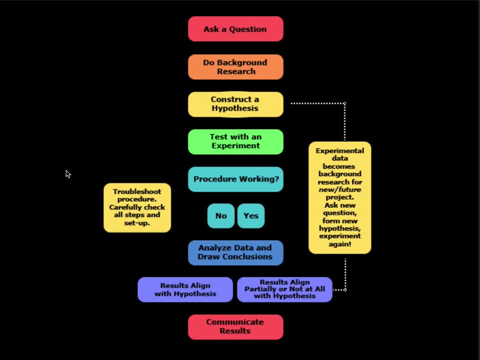 I am just going to jump straight to here. I want to test it. So what if I ask every student I meet How tall are you And what size shoe you wear? Well, I would need That would probably work For shoe size. it would be okay. 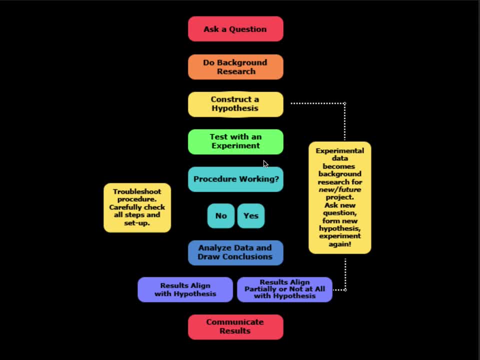 So I would get a lot of data. I am not talking like 20 people, I am talking about 300 at least. Then, if that data is working, Yes, I am going to analyze that data To try to come up with some solutions. 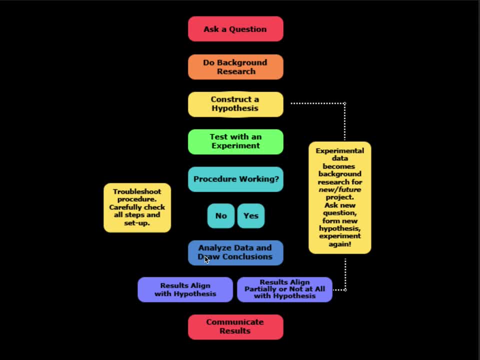 So what I would do is take that data And I would put it in Excel And I would create a trend line. I would plot it to see where everyone is, Then I would create a trend line And along that line I would get an idea. 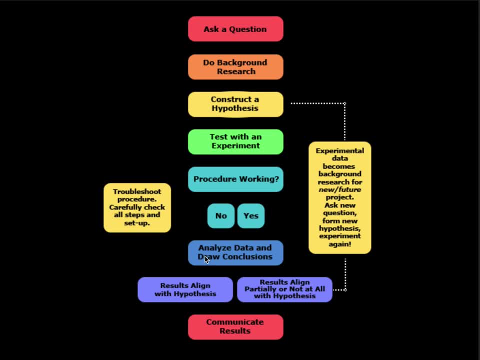 That okay, I am starting to see the taller people. Then how would I test my results? Well, I would, after I collect all my data, I would pick a random person And I would use just half of their data. Well, how tall are you? 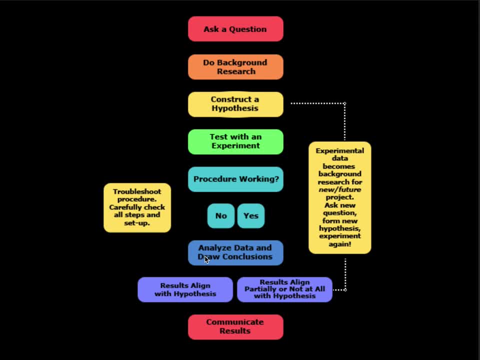 And then they would say: well, I am 5'11". Well then, I would plot 5'11 on my trend line. I would say: do you wear Size 10 and a half shoes? And they would go. well, I do. How did you know? 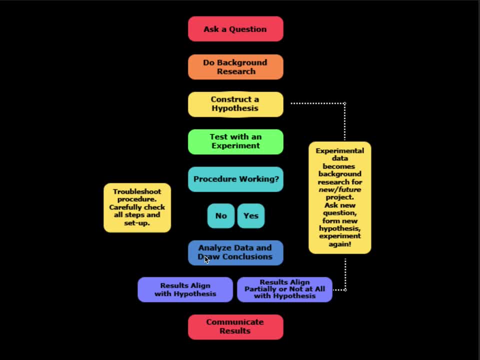 Then I would say: I tested my data And I think I can start thinking That this could be a true hypothesis. So then I would start checking other people Against my trend line And then I would either have to agree, I would have to accept. 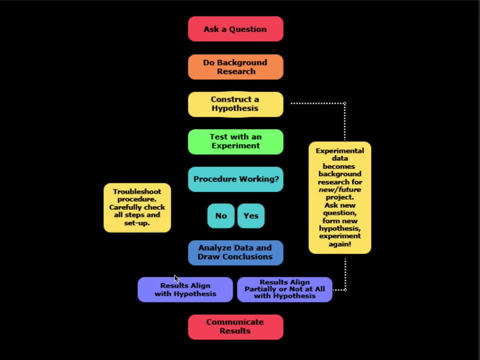 Or reject my initial hypothesis. If I accept it, Then I can communicate my results And then we can decide if this is a hypothesis That is going to work into a theory, Or if I reject it, I go back And let me tell you. 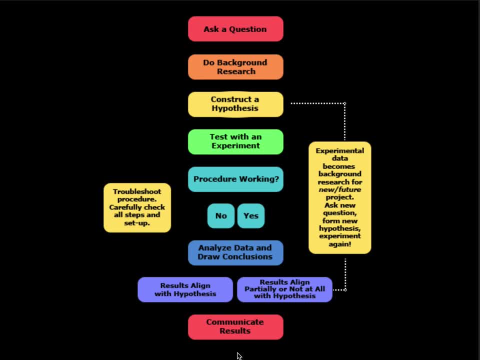 There is nothing better than rejecting your hypothesis. I know that sounds weird, But failure can be such a great experience Because, Hear me, You learn something, So you have results. I know that what I said was wrong, But I got some other results. 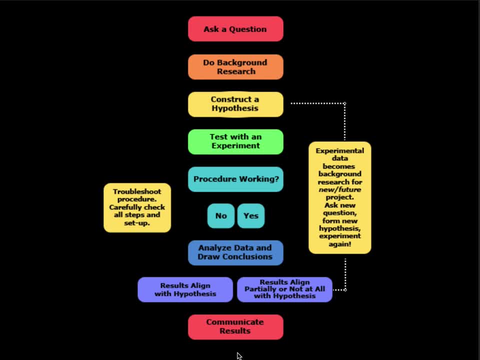 So how can I use those results To solve something new or different? Failure in science is so incredible Because it gives you the chance to do the work again And to try over and test new theories. That being said, Failure can also be negative.